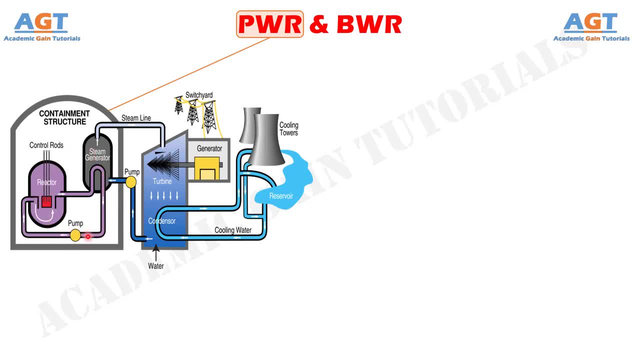 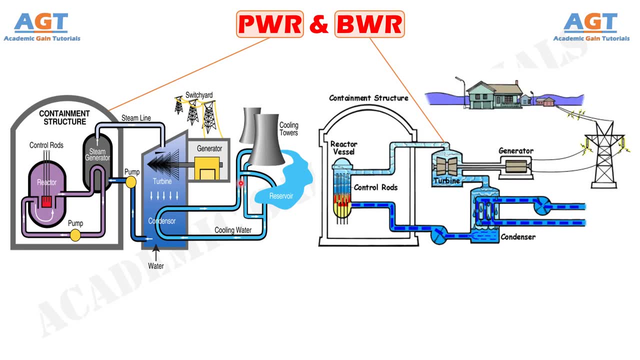 reactor, the primary coolant is pumped under high pressure to the reactor core, where it is heated by the energy released by the fission of atoms. On the other hand, a boiling water reactor is a type of light water nuclear reactor used for the generation of electrical power. 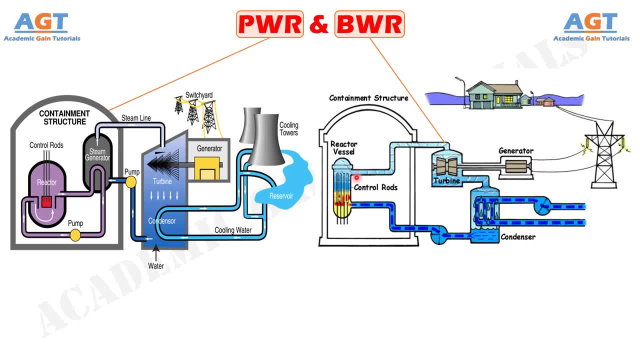 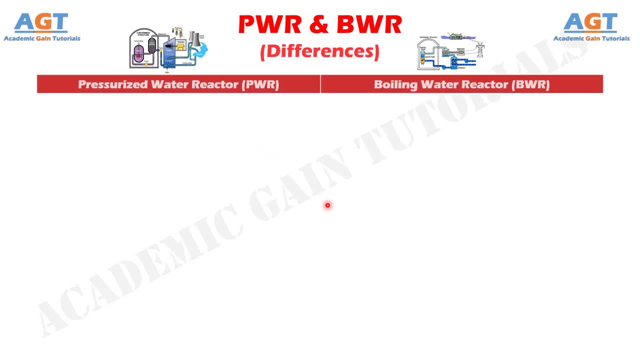 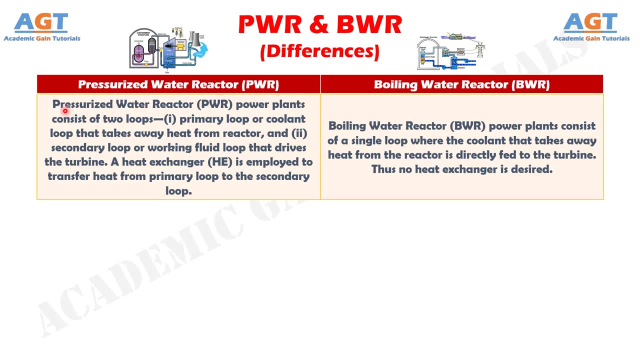 It is the second most common type of electricity generating nuclear reactor after the pressurized water reactor. So let's look into the basic differences between pressurized water reactor and boiling water reactor in a tabular form. Difference number 1.. Pressurized water reactor power plant. 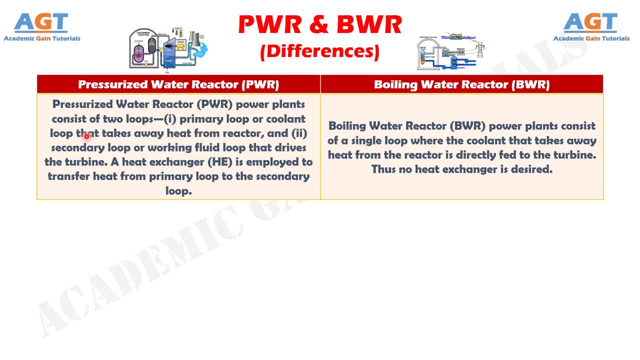 consists of two loops: the primary loop, or coolant loop that takes away heat from reactor, and the secondary loop, or working fluid loop that drives the turbine. A heat exchanger is employed to transfer heat from primary loop to the secondary loop, whereas boiling 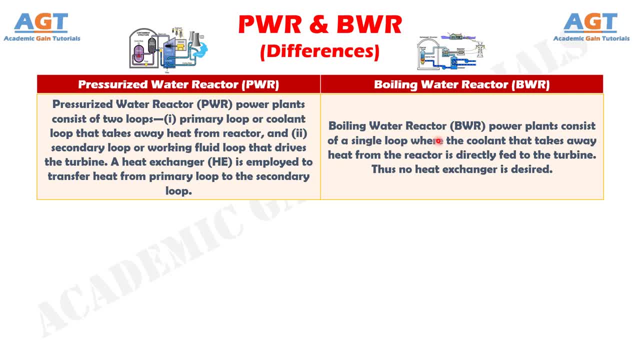 water reactor power plants consist of a single loop where the coolant that takes away heat from the reactor is directly fed to the turbine. Thus no heat exchanger is desired. Number 2. In the primary loop of pressurized water reactor there is no heat exchanger. In the primary loop of pressurized water reactor. 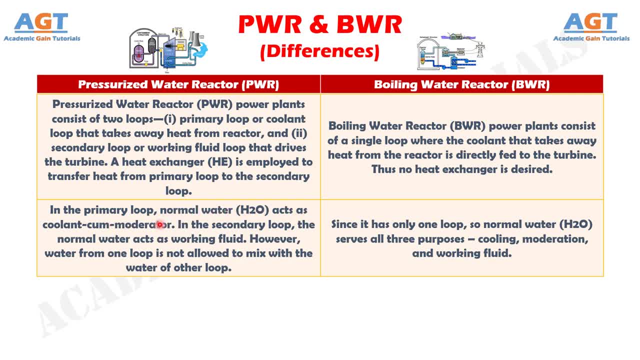 normal water acts as coolant-cum-moderator. In the secondary loop, the normal water acts as working fluid. However, water from one loop is not allowed to mix with the water of other loop, whereas since boiling water reactor has only one loop, so normal water. 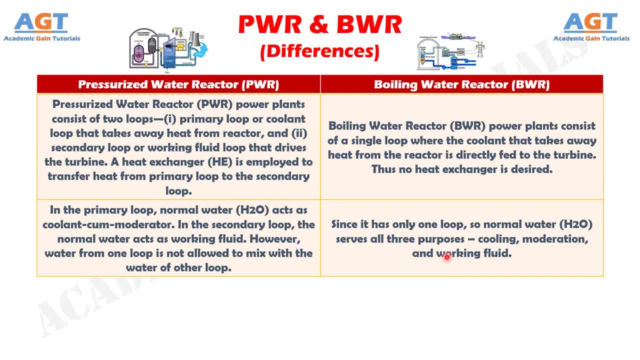 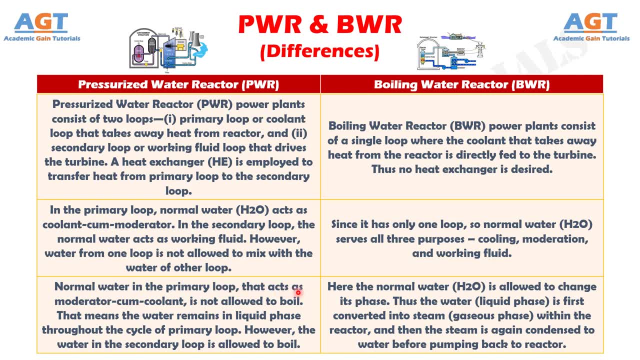 serves all three purposes: cooling, moderation and working fluid Number 3. Normal water in the primary loop of pressurized water reactor that acts as moderator-cum-coolant is not allowed In the primary loop of pressurized water reactor. 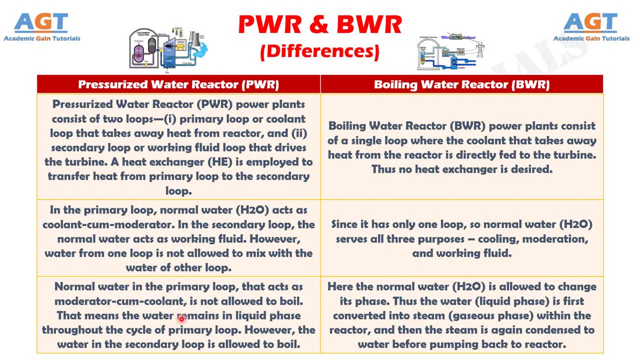 it is not allowed to boil. That means the water remains in liquid phase throughout the cycle of primary loop. However, the water in the secondary loop is allowed to boil, whereas in boiling water reactor the normal water is allowed to change its phase. Thus the water 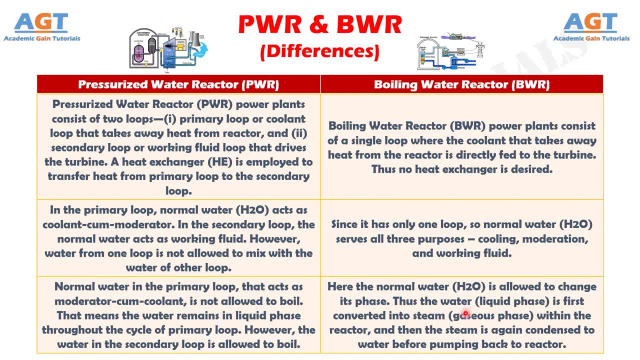 from liquid phase is first converted into steam at gaseous phase within the reactor, and then the steam is again condensed to water before pumping back to reactor Number 4.. In pressurized water reactor there is no heat exchanger In the primary loop. 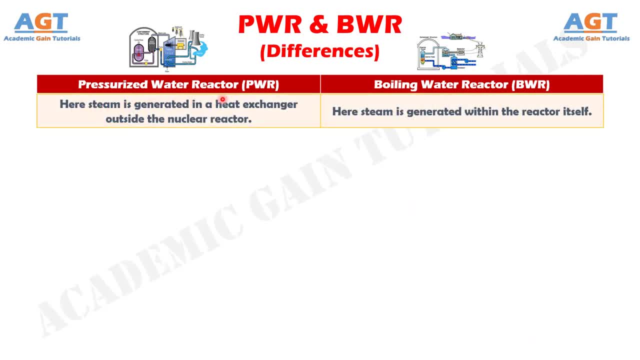 steam is generated within the reactor itself. Moreover, steam is generated within the reactor itself. Number 5. In pressurized water reactor power plants, the water in the primary loop is maintained at high pressure, about 15 to 17 MPa, to avoid boiling at reactor exit, whereas in boiling, 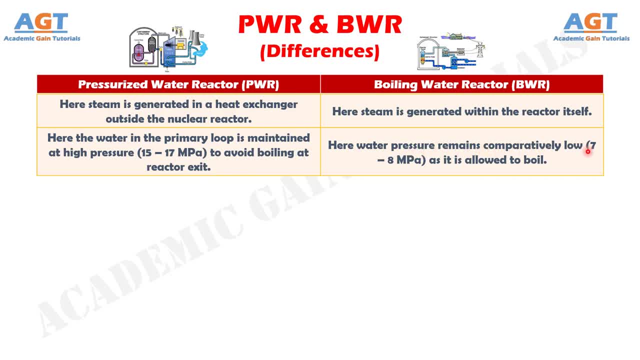 water reactor power plants, water pressure remains higher, comparatively low, about seven to eight megapascals, as it is allowed to boil. number six: in pressurized water reactor, a pressurizer is required to use mandatorily to maintain water pressure in such a way that it does not evaporate. 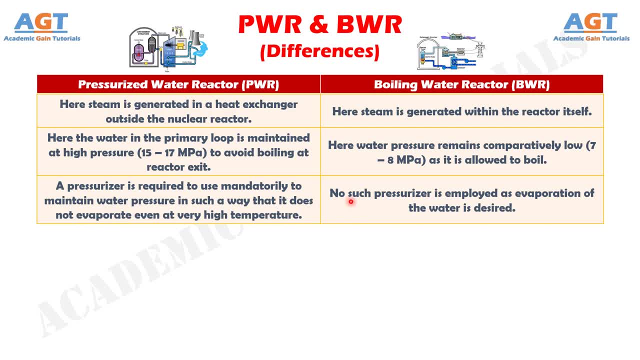 even at very high temperature, whereas in boiling water reactor power plants no such pressurizer is employed, as evaporation of the water is desired. number seven: the temperature of the water at the pressurized water reactor exit is kept around three hundred and ten degrees centigrade, corresponding to 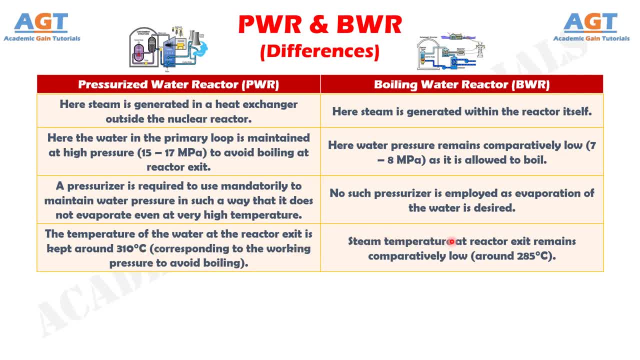 the working pressure to avoid boiling, whereas steam temperature at boiling water reactor exit remains comparatively low, around two hundred and eighty five degrees centigrade. number eight: pressurized water reactor has comparatively low thermal efficiency owing to two different loops, whereas boiling water reactor offers higher thermal efficiency. number nine in: 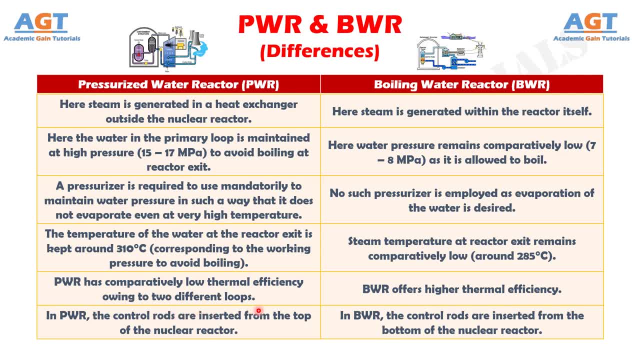 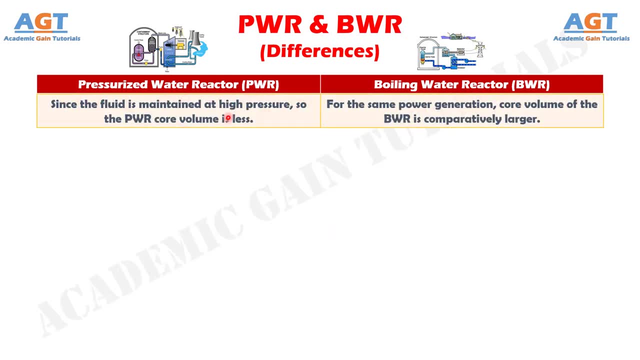 pressurized water reactor the control rods are inserted from the top of the nuclear reactor, whereas in boiling water reactor the control rods are inserted from the bottom of the nuclear reactor number 10, since the fluid is maintained at high pressure. so the pressurized water reactor core volume is less, whereas for the same. 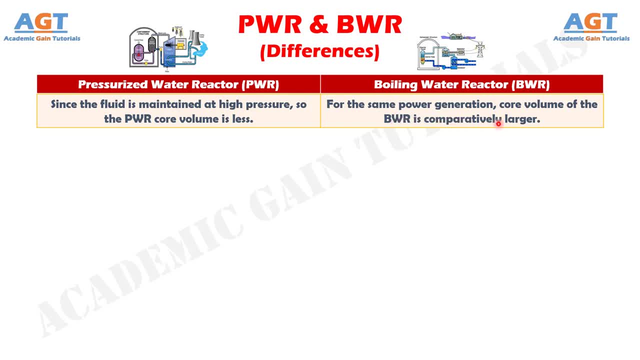 power generation. core volume of the boiling water reactor is comparatively larger and difference number 11, since the working fluid loop is separated from the primary loop. so pressurized water reactor is less risky in spreading of radioactive materials owing to leakage, whereas since same fluid passes through. 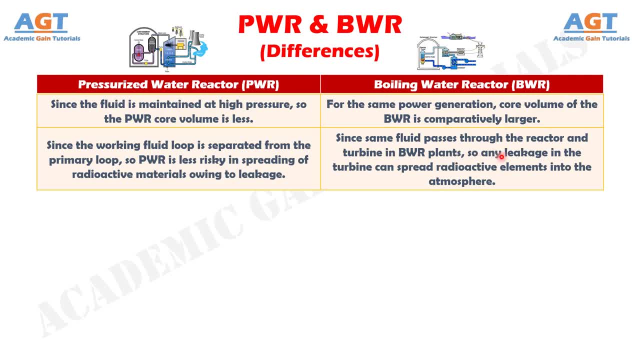 the reactor and turbine in boiling water reactor plants, so any leakage in the turbine can spread radioactive elements into the atmosphere.